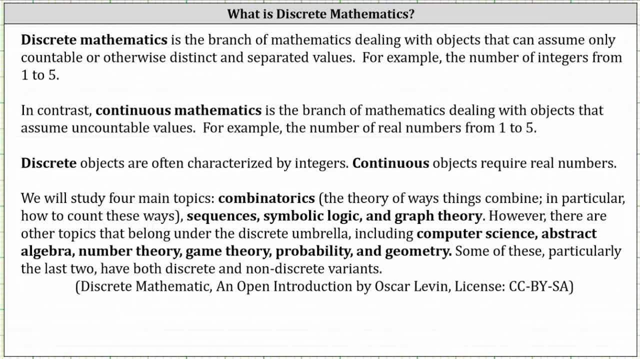 What is discrete mathematics? Discrete mathematics is the branch of mathematics dealing with objects that can assume only countable or otherwise distinct and separated values, For example the number of integers from one to five. In contrast, continuous mathematics is the branch of mathematics dealing with objects that assume uncountable values. 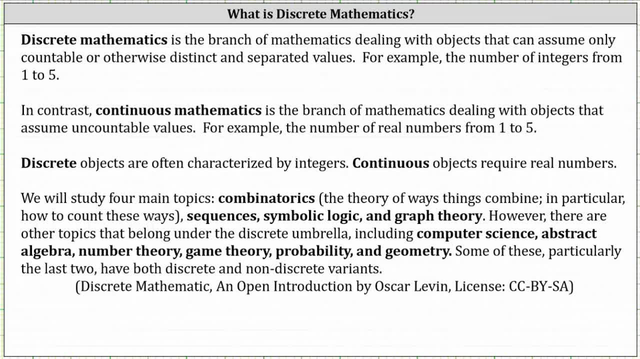 For example, the number of real numbers from one to five. Remember, there are an infinite number of real numbers, from one to five. Discrete objects are often characterized by integers. Continuous objects require real numbers. We will study four main topics: Combinatorics. 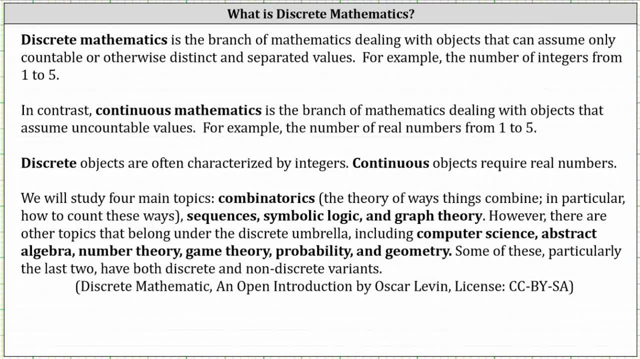 which is a theory of ways things combine, In particular how to count these ways, Sequences, symbolic logic and graph theory. However, there are other topics that belong under the discrete umbrella, including computer science, abstract algebra, number theory, game theory, probability and geometry. Some of these, particularly the last two, 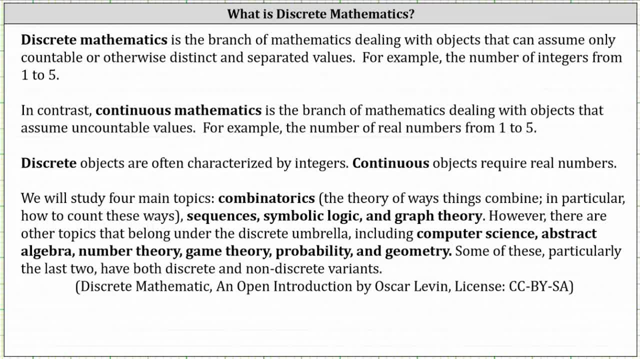 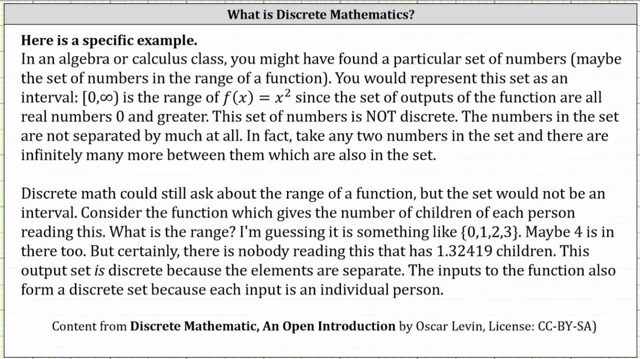 have both discrete and non-discrete variants. Let's take a look at an example. In an algebra or calculus class you might have found a particular set of numbers, maybe the set of numbers in the range of a function. You would represent the set as an interval, For example. 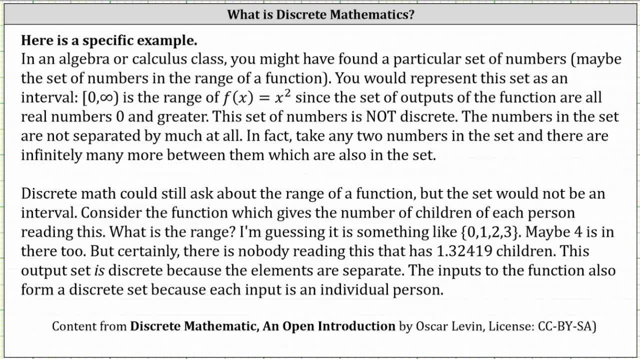 the interval from zero to infinity, where the interval is closed on zero and open on an infinity, is the range of the function. f of x equals x squared. since the set of outputs of the function are all real numbers, zero and greater, This set of numbers is not discrete. 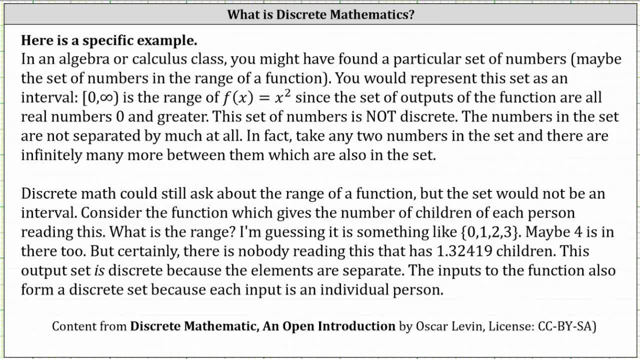 The numbers in this set are not separated by much at all. In fact, take any two numbers in this set and there are infinitely many more between them, which is also in the set. Discrete math could ask about the range of a function, but the set would not be an interval. Consider the function. 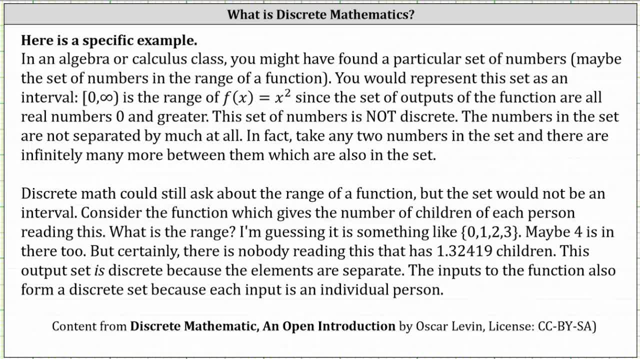 that gives the number of children for each person reading this, What is the range? I'm guessing it is something like the set containing 0,, 1,, 2, and 3.. Maybe 4 is in there too. Certainly there is.